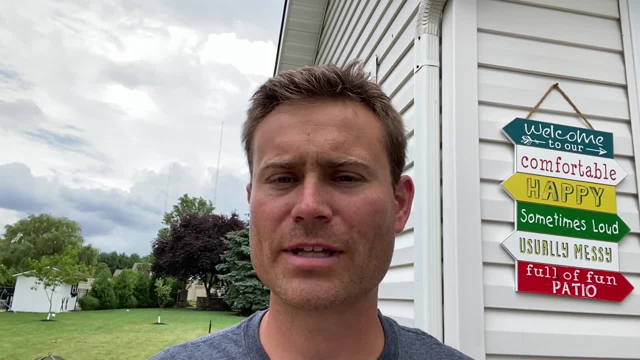 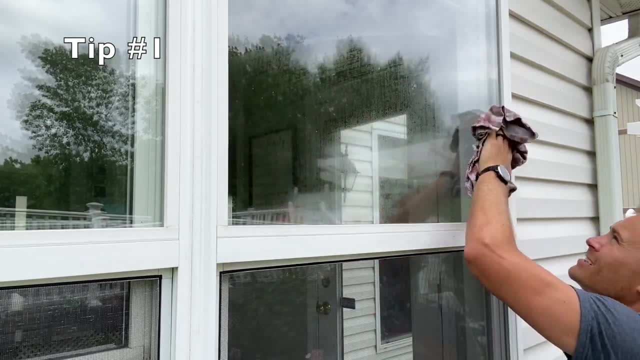 that the suction cups on your window bird feeders stick well to your window, so you'll never have it fall, okay? so the first thing you need to do is make sure you clean the window. I know this seems obvious, but a lot of people, including myself, forget to wash the window. and if the window is 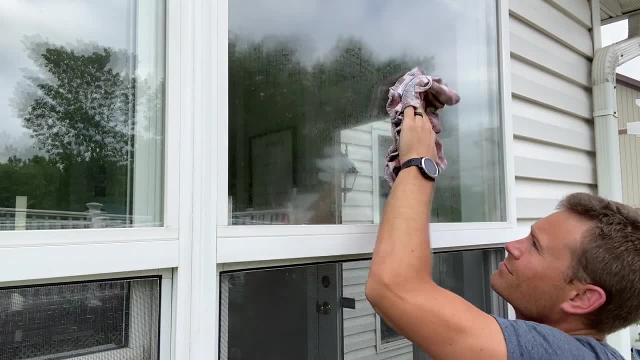 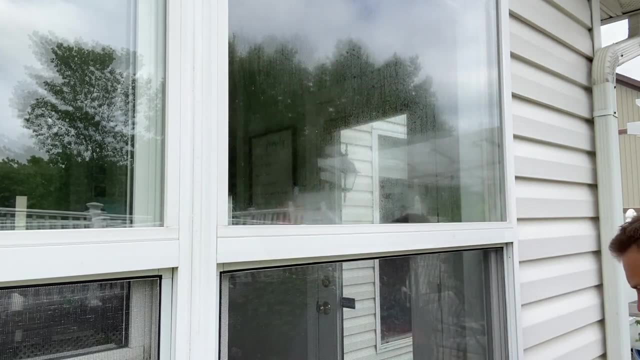 dirty, it can be hard to clean the window, so I'm going to show you how to do that. It's hard for the cups to get a good suction onto the window. now here's the thing: make sure you don't use any soap when you clean. the soap can leave a residue. 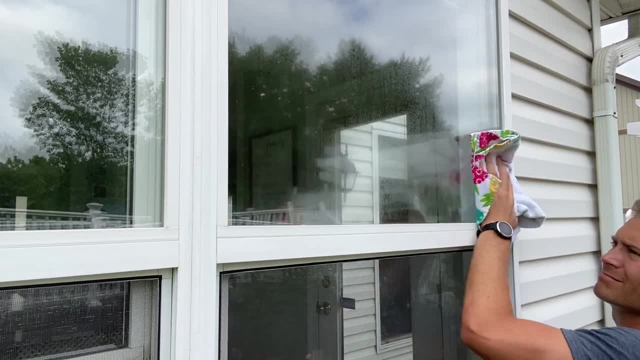 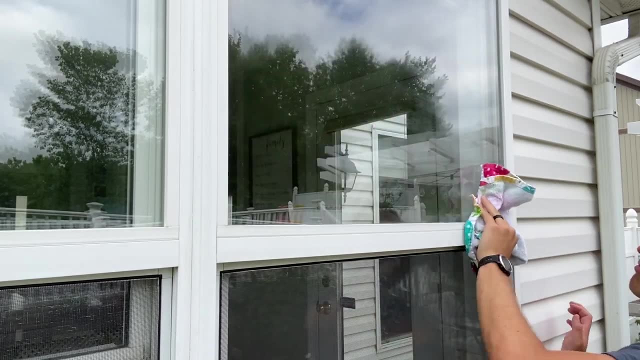 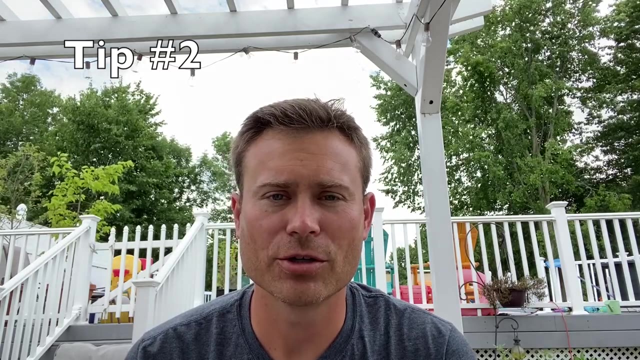 on the window that the suction cups can't grasp or suction onto. so just take a wet rag, wash the window and then dry, all right. the second way to make sure your window bird feeder stick to your window has to do with the actual suction cups on the feeder. so I'm using a hook. 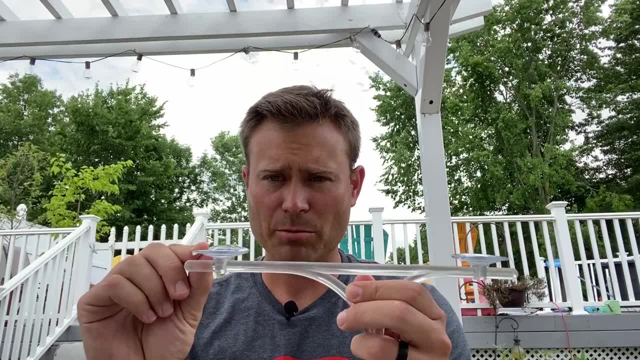 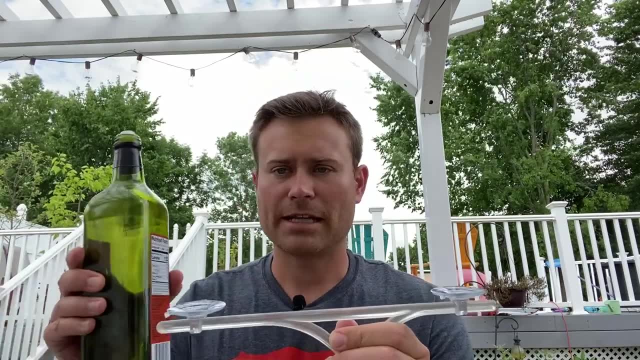 today which I hang a feeder from. but obviously the suction is really important. not a good suction, it's going to fall to the ground. so to make sure you have a great suction, take some oil. this is olive oil from my kitchen. get the tiniest bit on your finger, I mean. 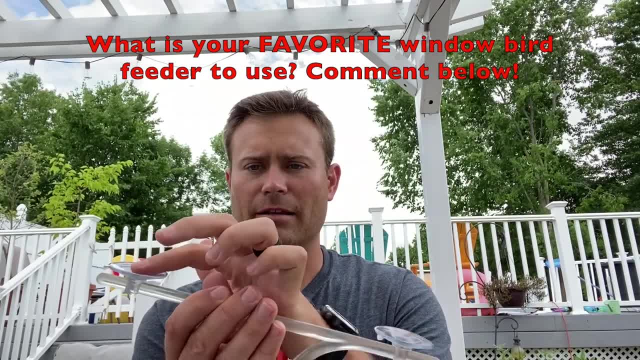 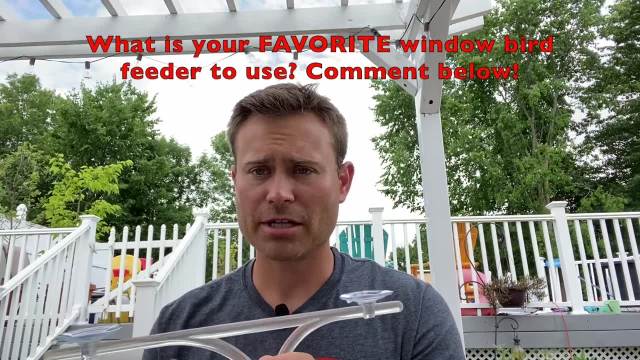 the smaller the better, and rub it on the suction cup, just like that you don't have any olive oil or cooking oil in your kitchen and what actually? what I usually do is there's enough natural oil found on your face. if you wipe my forehead, or some people wipe their, 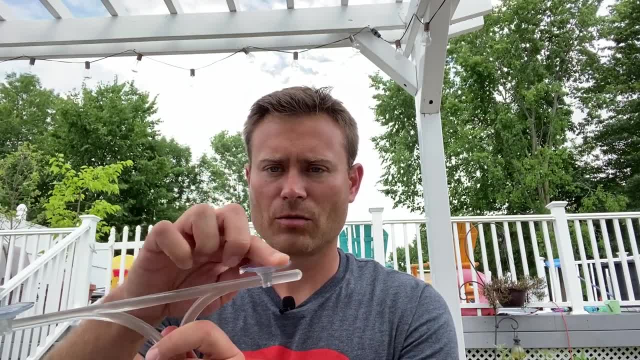 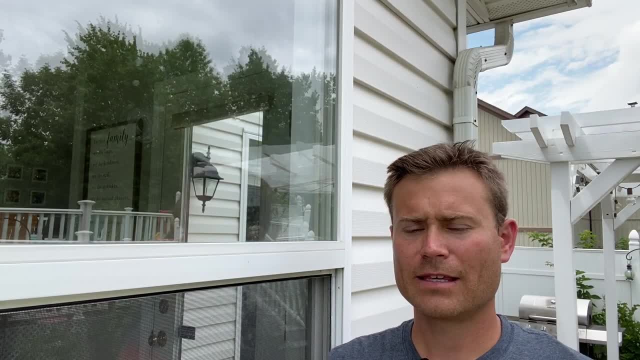 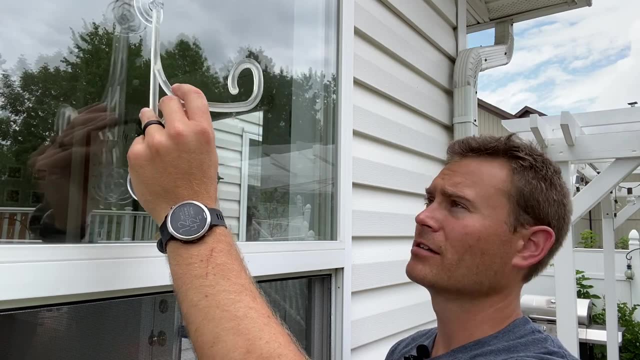 nose, use the other suction cup and rub it right there. that is all you're going to need now. watch this. okay, now that we've got the little bit of oil on our suction cups, I'm going to show you how to get it back onto the window. so, really, from here, just take your feeder and put it on and 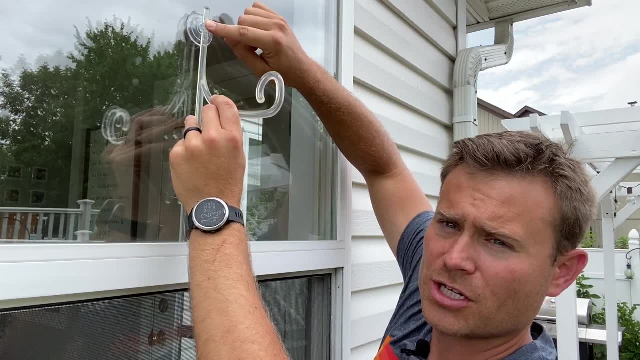 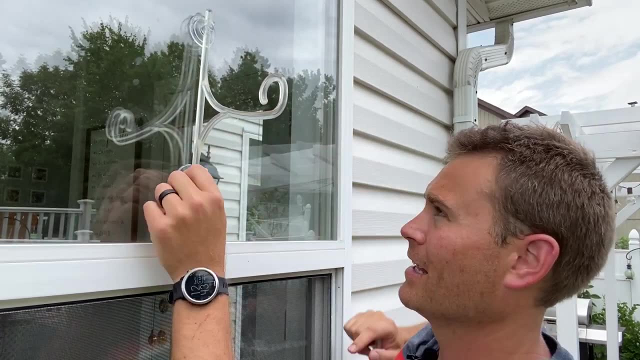 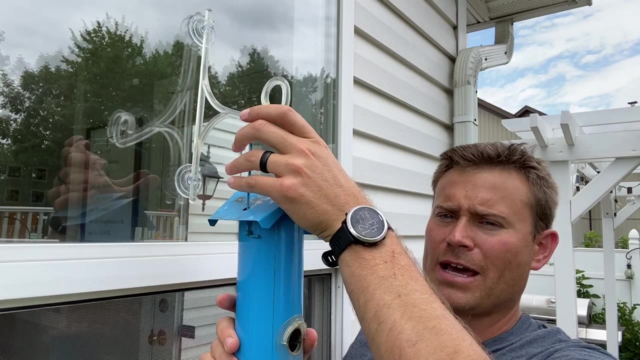 here's what's important: make sure what really gives it an awesome suction is that you push right in the center. see that, and right here, right in the center, that just gives an awesome, excellent, strong hold. lastly, we'll take our feeder, put it back on the window and look at that.